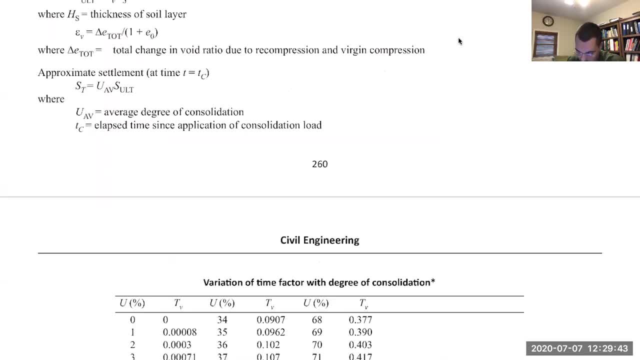 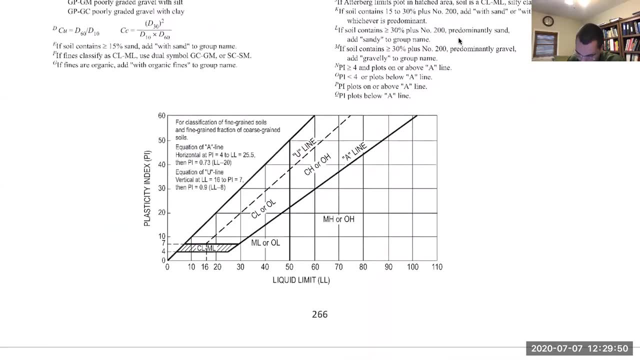 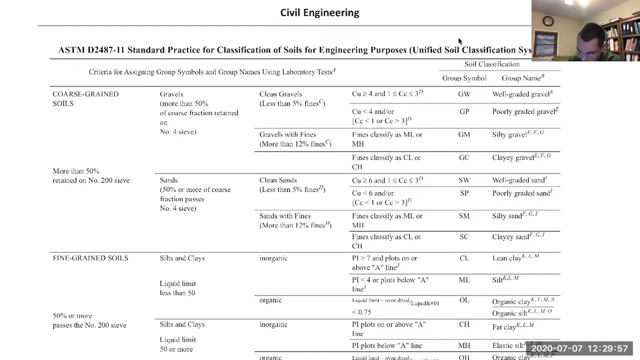 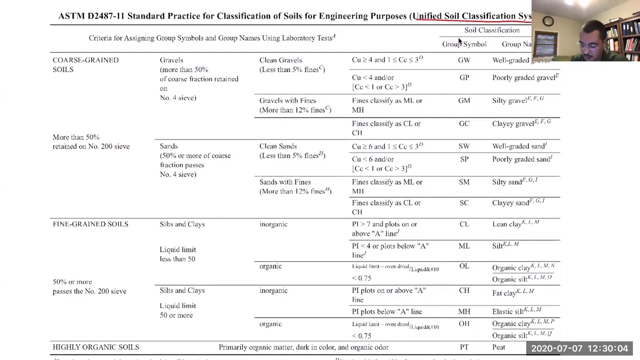 and added more pages so that everything fits in nicely. So if we go to page 226 on the FE manual, again, it's the 10.1.0.1 manual. We're going to look here at the Unified Soil Classification System, or USCIS. 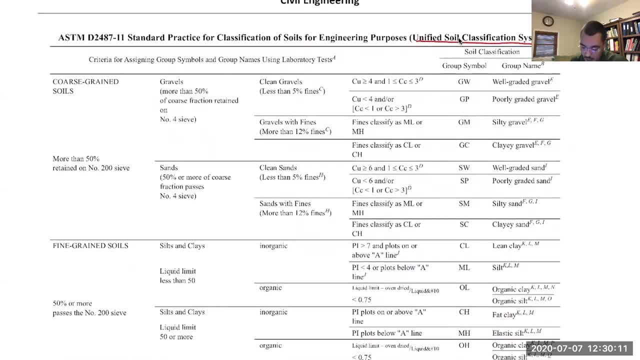 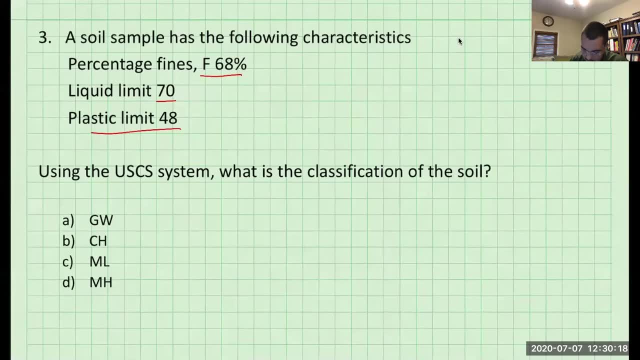 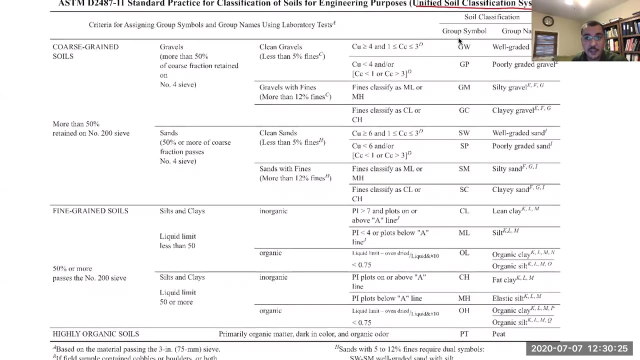 So that's the Unified Soil Classification System. Now, in our particular question, we have, if I remember correctly, okay 68% fines. So here, how do you use this soil classification system? You always start on the left-hand side and keep going forward. 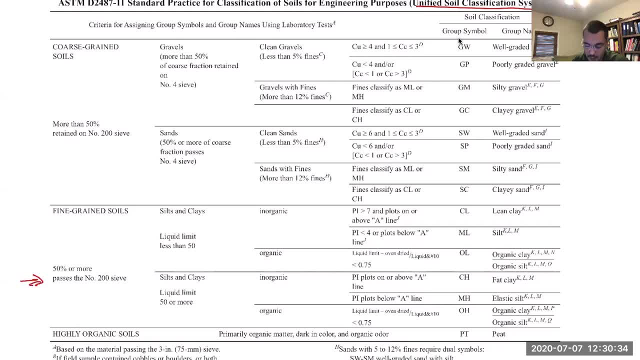 And see: is this in your givens or not? So, for example, we have here 50% or more passing the number 200 sieve And we know that the number 200 sieve defines anything passing that defines our fine portion. So we have 68% passing the number 200 because the question told us that we have 68% fines. 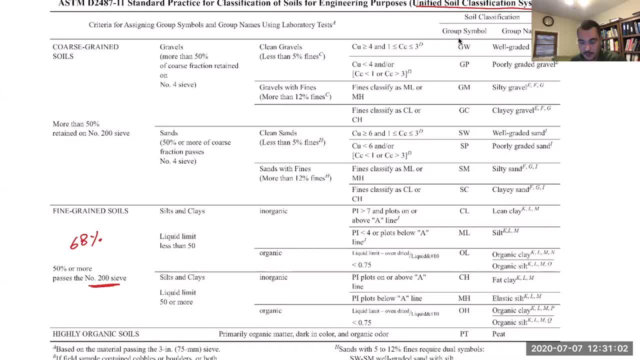 which means fines. Those are passes. So we're passing the number 200 sieve And now we go to the right side and we look at what is the criteria. here We have a liquid limit less than 50 or a liquid limit 50 or more. 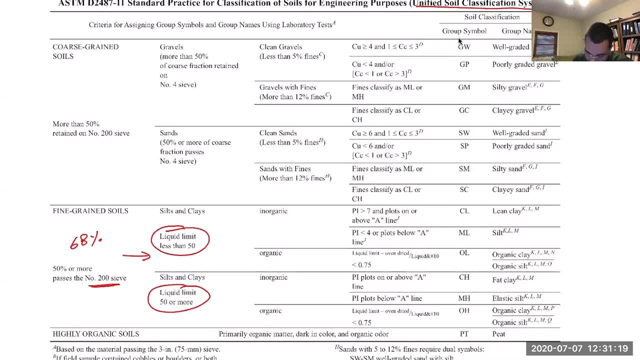 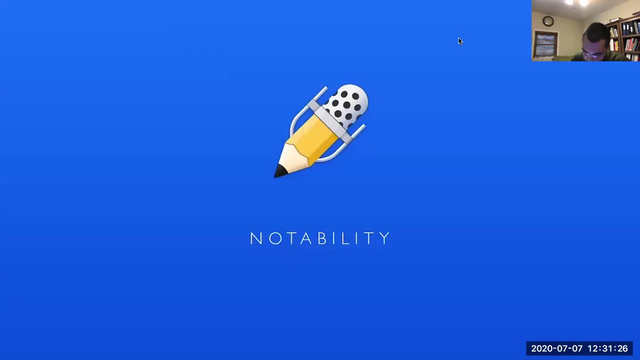 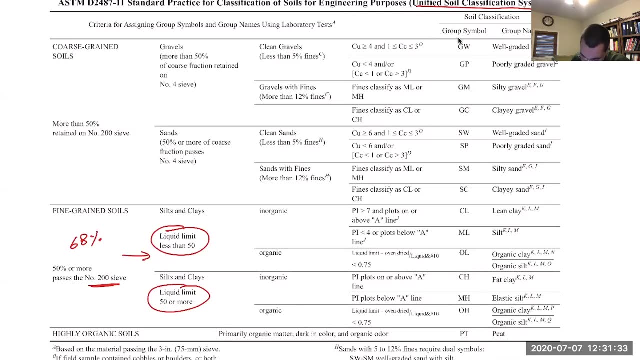 Now in our question the liquid limit is 70. So right here it's 70. So we keep going forward. So the liquid limit is 70.. The liquid limit is 70. So it's 50% or more. 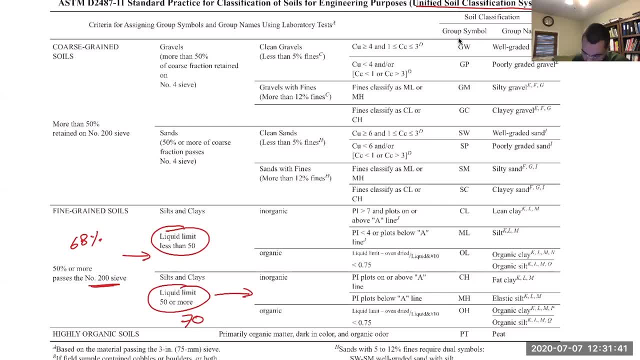 Now we continue to the right side, So we're not in this area, We're at the bottom portion. Now, here you have inorganic or organic, So take note. if the question says something about having organics, then you need to take. 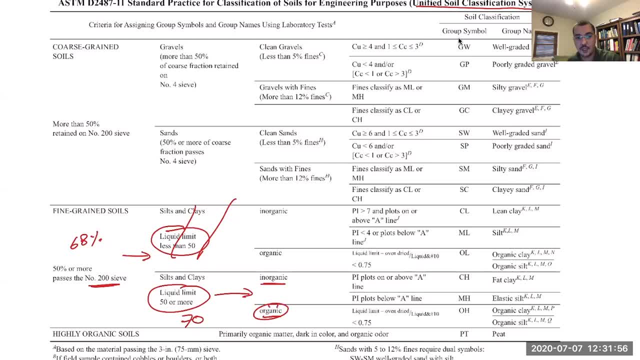 a look at this side. But because our question did not mention organics, we're going to assume that it's inorganic. Okay, now we keep going to the right side. now it says here: PI plots on or above line A or the PI plasticity index plots below line A. it's either a CH, so clay high. 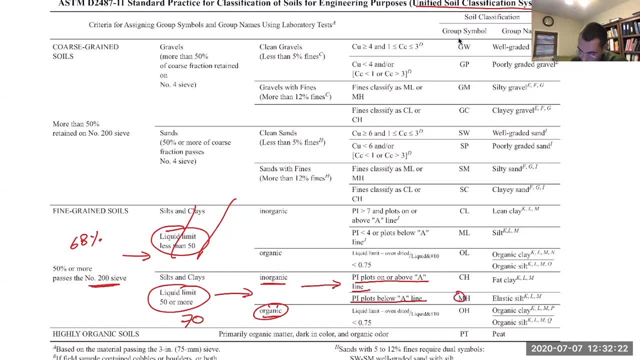 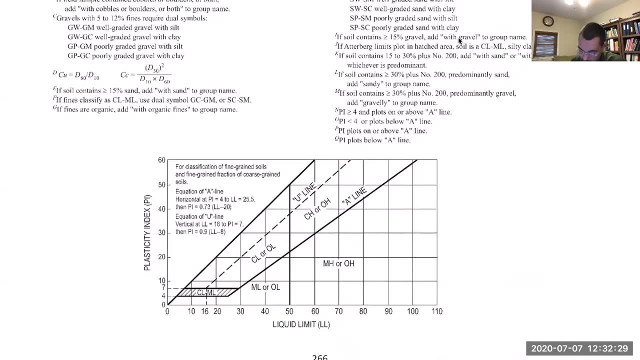 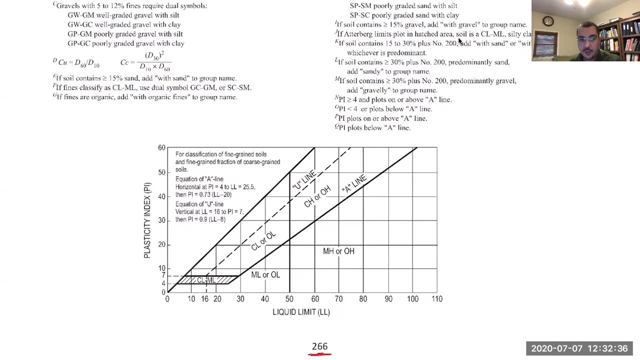 plasticity, or silt. M refers to silt, silt, high plasticity. now, what is this chart that they're referring to? this chart is right here. it's a Casagrande chart and it can be easily used to classify soils. so in our particular case, we have a 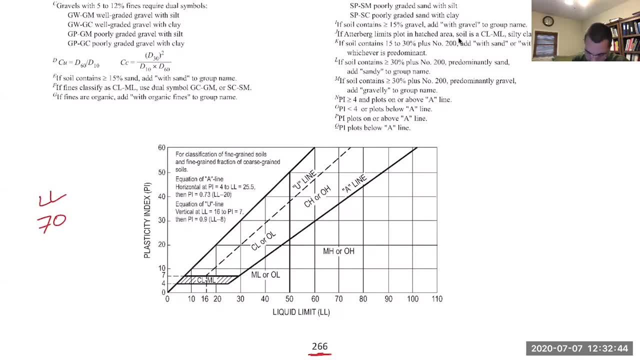 liquid limit of 70. that's our liquid limit and we have a plastic limit of 48. so right here to enter the chart, we need the plasticity index, and the plasticity is equal to the liquid limit minus the plastic limit, and so we have 70 minus 48. 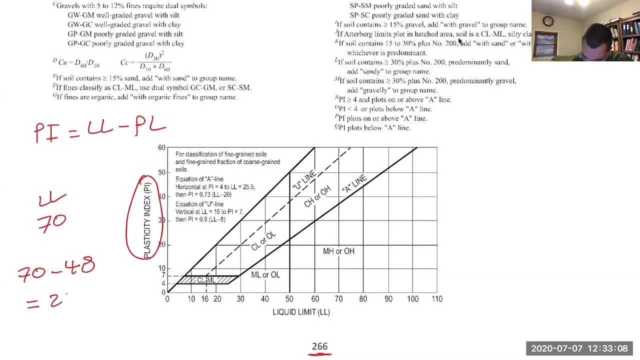 and that's equal to 22. and so now we can enter the chart because we have the liquid limit and we have the plasticity index and remember, this chart is for fine-grained soils. so we go from the X- Y axis straight with a straight line and 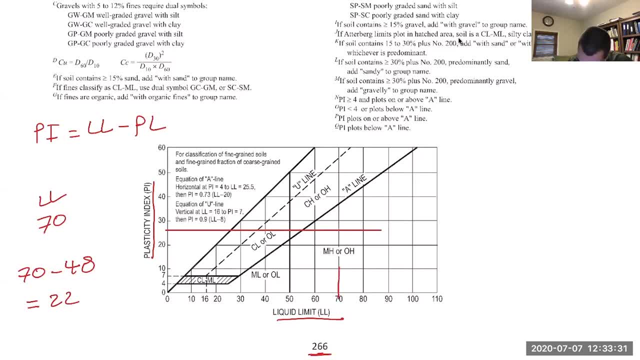 then from the 70, which is our liquid limit given in our question, we see where do we fall. so we fall in in. if you imagine this as being a whole quadrant, this is it right here. this is a quadrant. so now and like, let me try this, maybe so. 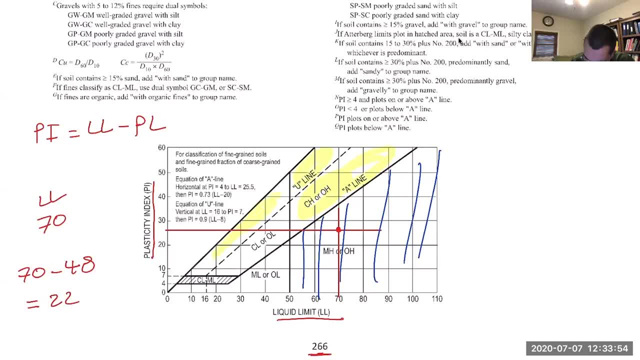 see, here, there's a quadrant, here, there's a quadrant here, there's a quadrant here. and remember, and it said that if the plots below line a, so this is line a right here, correct, this is line a, and we plot below line a. so again, O stands for organics and we